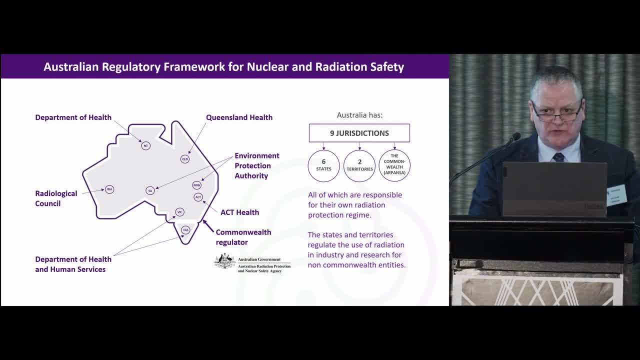 so we have the Commonwealth regulator. we're actually in every jurisdiction, we have all the states and territories, so we're actually everywhere and the each state and territory has their own act and regulations and- sorry, I don't know what happened there- they have their own act and regulations which they use for. 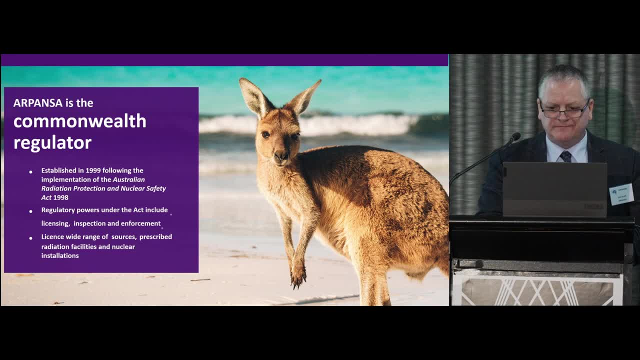 regulation. so our Panzer was actually established in 1999, with the the our Panzer act being established and then the regulations- sorry, the our Panzer act- in 1998 and then followed by the the our plans regulations in 1999. now we are an. 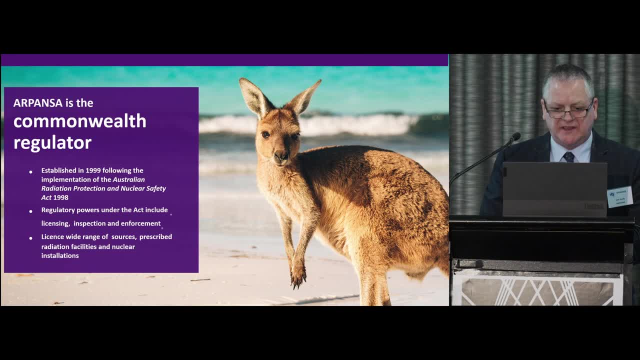 independent regulator, and I'd like to tell you a little bit about this independence. in fact, prior to 1998, the only research reactor in Australia at the time was the was the, the high far 10 megawatt diro reactor, and it was regulated by the nuclear safety Bureau, which 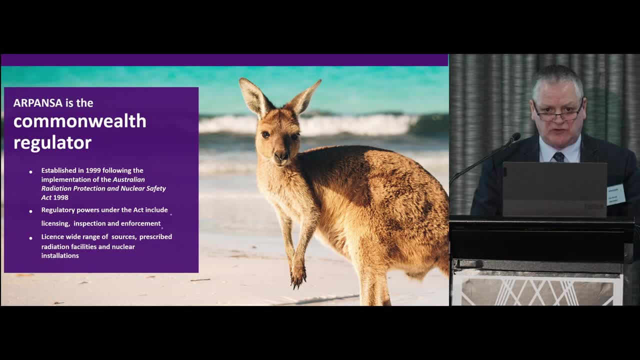 was an internal regulator embedded in the ANSTO organization. however, with the research reactor replacement project, which was to become Opal, the government's intention was to move best practice, which was to have an independent regulator, and so hence a Panzer, come into being. it was. 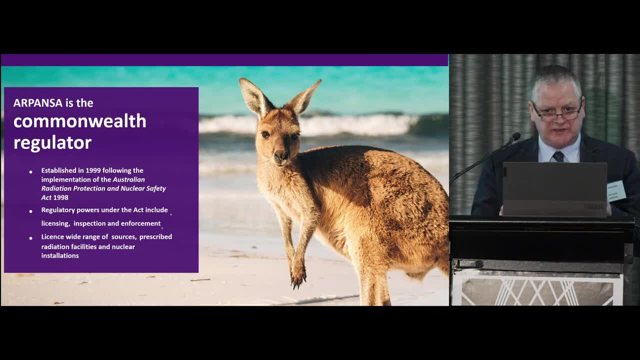 actually a formation of two organizations: the nuclear safety Bureau, which was the, the ANSTO regulator, and the Australian radiation laboratories, which were based in Melbourne. so it was actually a merger of two organizations and we came into being- but notice the independence part- that we weren't. 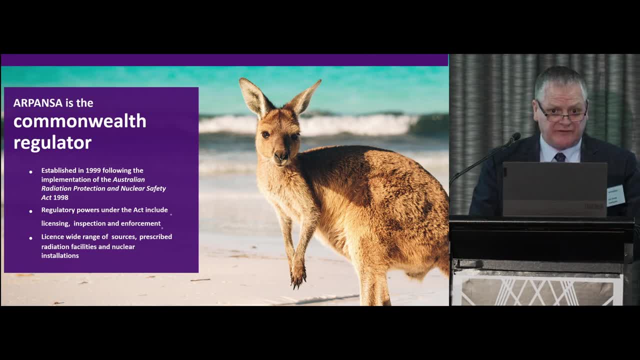 part of the operator. we have uh independent from all of our of our license holders. so we have an action regulations and our regulatory powers include issuing licenses, undertaking inspections and enforcement actions. uh, we, we license a wide range of things. I'll try to concentrate on the nuclear installations because 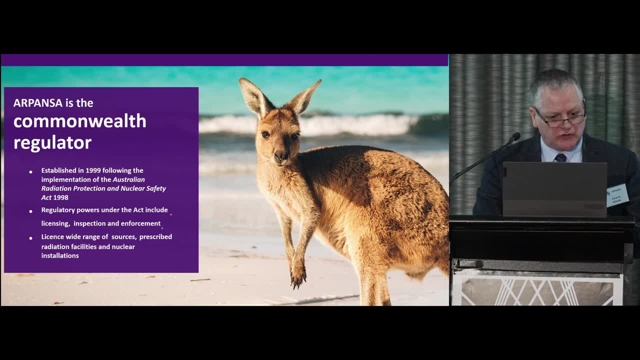 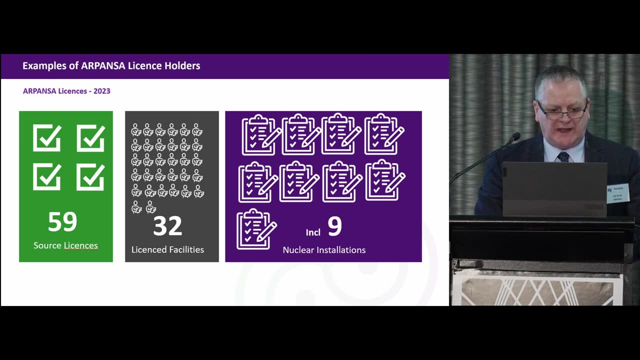 this is a nuclear conference, but we, we license sources, prescribed radiation facilities and nuclear installations. so who do we regulate? so? uh well, what do we regulate? so we've actually got 59 source licenses, 32 licensed facilities and nine nuclear installations. all of those nuclear installations are actually operated by the ANSTO organization. uh, Lucas heights, and in fact the majority of our. 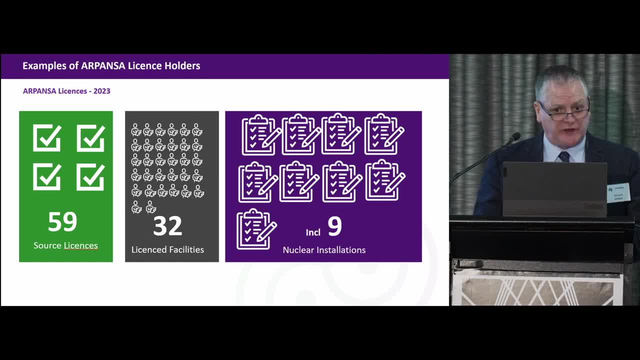 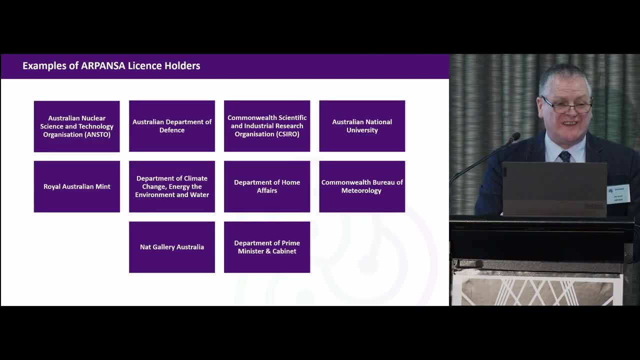 licensed facilities. over 20 of them are actually operated by ANSTO, so ANSTO is a very large part of our business. uh, okay, so example of licence holders that we regulate: Well, we actually regulate 30 Commonwealth organisations that use radiation And in 21,, 22, the financial year, we had said 30 organisations. I've just 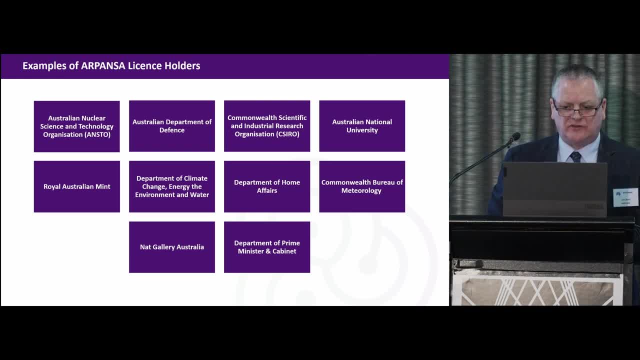 given you a snapshot of some of the larger of these organisations, namely ANSTO, who are a sponsor for this conference, the Australian Department of Defence and, of course, there's a lot of discussions going on about nuclear submarines. So the Commonwealth Scientific 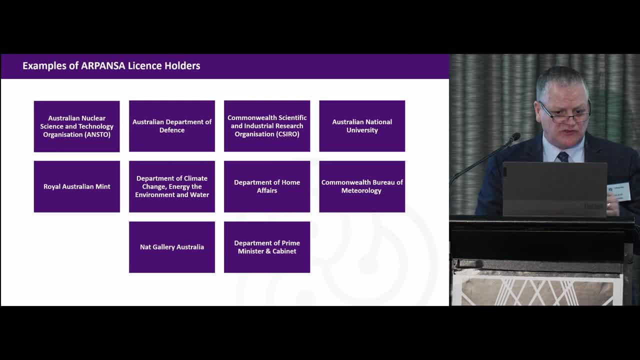 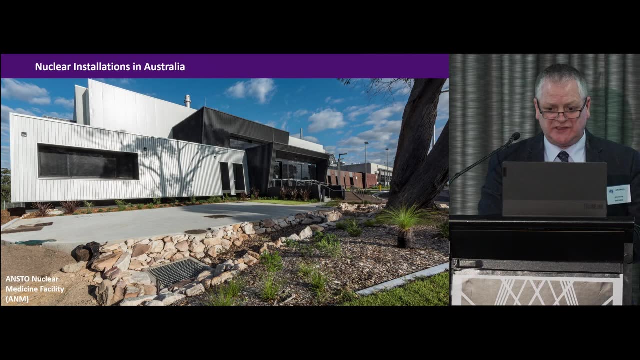 and Industrial Research Organisation, the Australian National University, and you can see them there. That's just a snapshot of the examples. So the ANSTO organisation has nine nuclear installations which we regulate. So these are examples. So here in front of me is the ANSTO Nuclear Medicine Facility which we 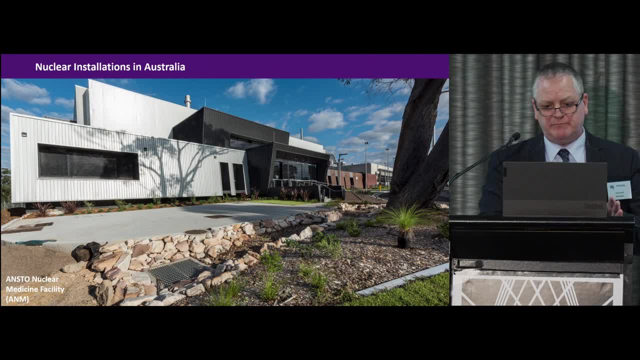 normally regulate. It's referred to as the ANM Facility, which makes radiopharmaceuticals for medical treatments, radiotherapy and also diagnostic imaging in Australia. So the nine nuclear installations that are actually regulated by us are research reactors, waste stores and radiopharmaceutical. 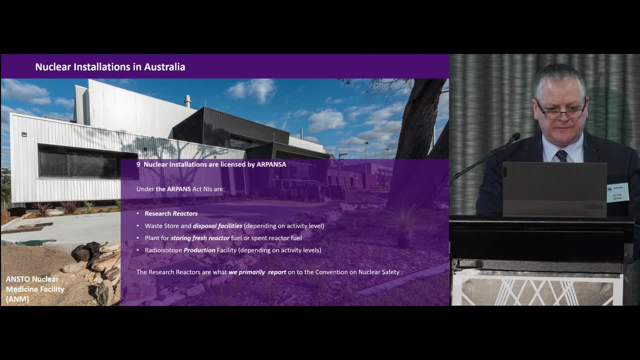 production facilities. So the research reactors, well, of course, there was the original Moata 100 kilowatt argonaut type reactor, which has been decommissioned and dismantled, And then the high-far 10 megawatt dyno type reactor, which operated from, I think, 1958 to 2007.. The OPPO reactor, 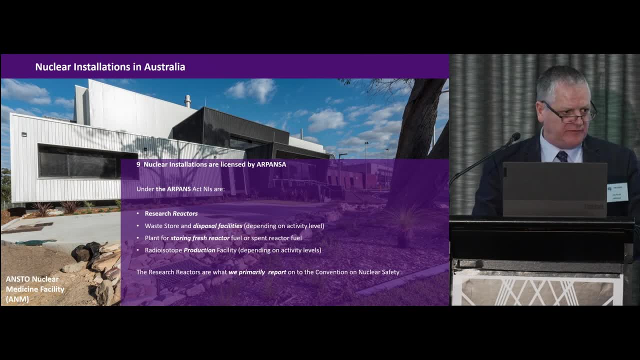 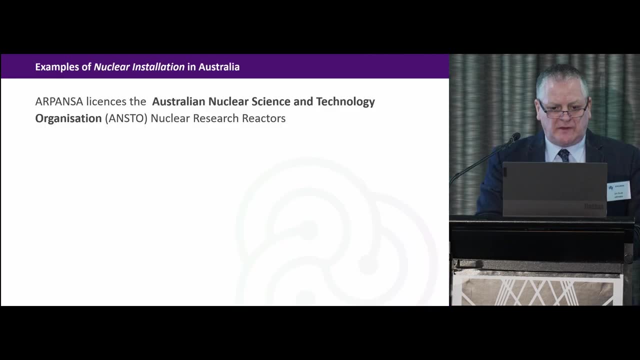 was basically formally opened in 2007 by the Honourable John Howard, which was the first one to be mentioned in a previous presentation. So these are the reactors: the 10 megawatt dyno type reactor. It's a bit interesting. 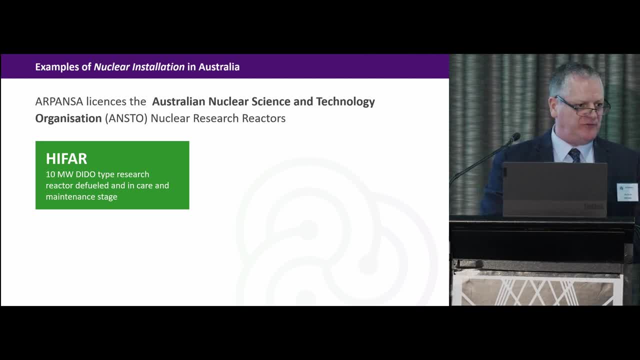 I have a little bit of when I worked at Harwell when I was a student back in the UK, and when I first walked onto the site I said, oh, I recognise that It was exactly similar to the dyno reactor. Well, it was the dyno reactor at Harwell, So it sort of reminded me of my 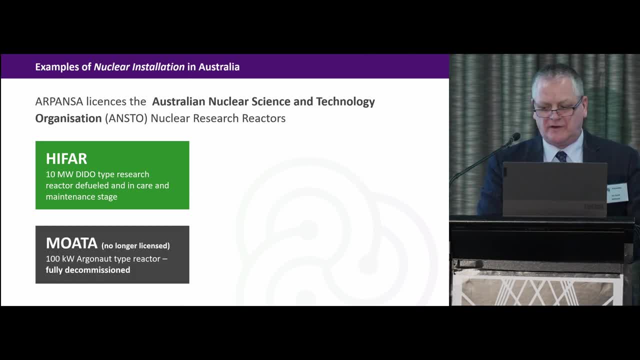 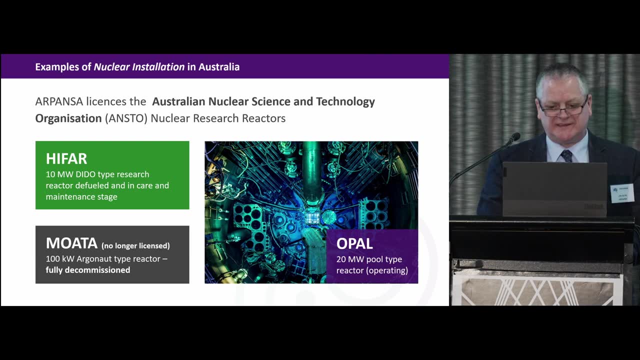 student days. And then Moata, which is obviously no longer licensed and it's an argonaut type reactor, of which there are many over the world. And then, of course, the new, latest and greatest OPPO reactor which has been effectively, was commissioned in 2006 and formally opened. 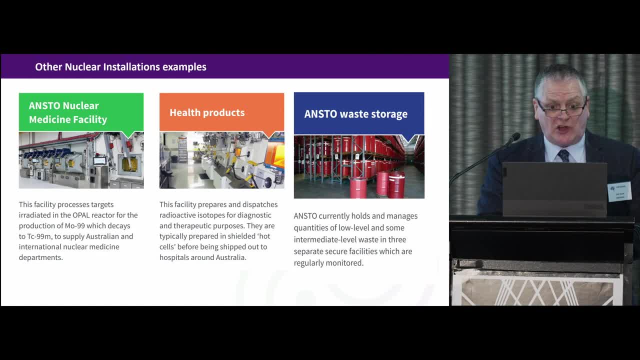 in 2007.. So other nuclear installation examples: well, as I said, there's the A&M facility, which we regulate. in this image in the top left, It shows you the front of hot cells- where they're in the front of hot cells. And then there's the OPPO reactor, which is the 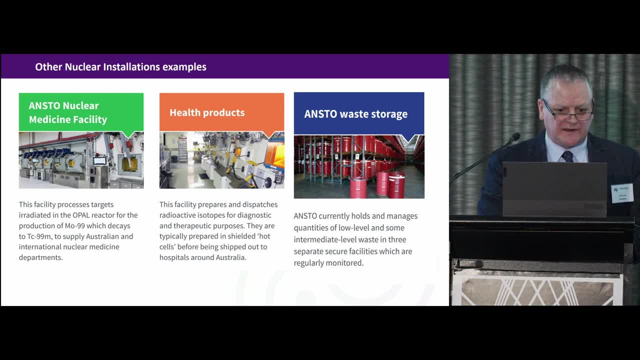 actual targets from the OPPO reactor are effectively reprocessed and the molybdenum extracted for supplying to hospitals and clinics throughout Australia. I'm also a former nuclear medicine physicist, so I've used these generators, these GenTech generators and the isotopes. 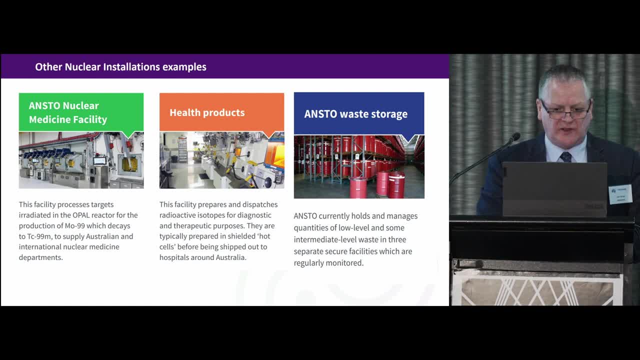 that Anstol makes. And then there's the health products, the Anstol health products, which make up the radiopharmaceutical kits for diagnosis and treatment of cancers, For example lutetium-177 for prostate cancer and neuroendocrine tumours, and radioiodine. 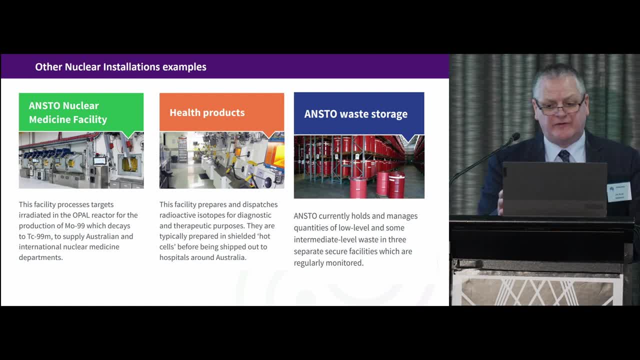 for treatment of thyroid cancers and diagnostic imaging. And then, of course, let's not forget the waste, because the waste is. you know, every nuclear activity will generate radioactive waste. And of course, Anstol has got licences for storage of waste at the locusite site. 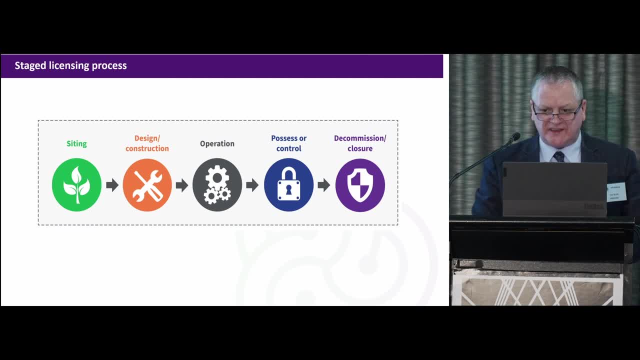 So a little bit about the stage licensing process that we have. So we, in alignment with international best practice, we issue licences on a stage basis, starting from siting to construction and design, operation, possessor control and ultimately to the end-of-life decommissioning, And in fact there's a lot of facilities that are. 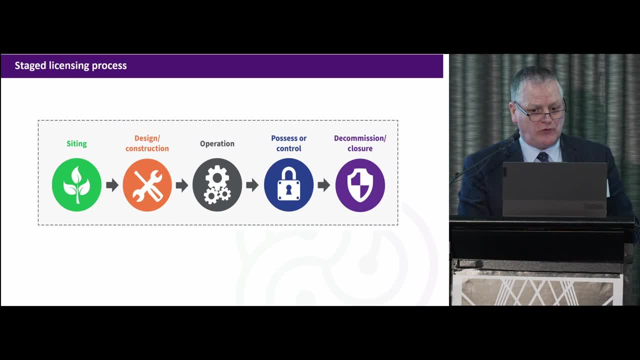 currently at that decommissioning stage at the moment. Now I will tell you about a public forum that we're having this Monday at 6pm. Thank you, You can find some details about it on the Urpansa website. We're having a public forum. 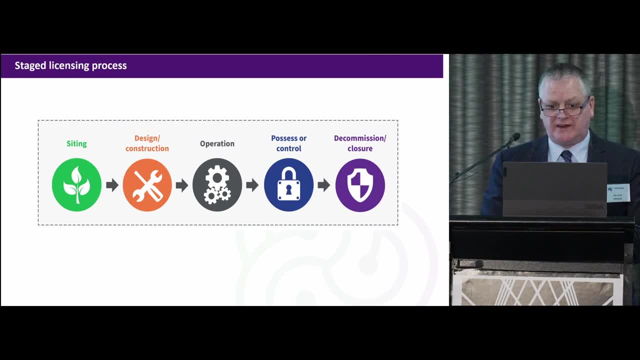 on the decommissioning of Phase A for the HIFAR reactor, and I would encourage you to join if you wish to find out more about the HIFAR decommissioning. It will be hosted by both CEOs, Sean Jenkinson, from the CEO of Anstol, and Dr Gelliner, the CEO of Urpansa. 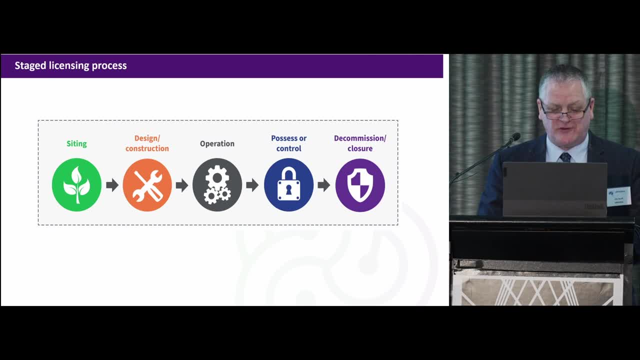 So that's at 6pm on Monday, this Monday coming. so have a look at the website. So why do you do a staged licensing process? It's a bit interesting because the safety case for any nuclear installation is an evolving document, It's an evolving set of arguments. 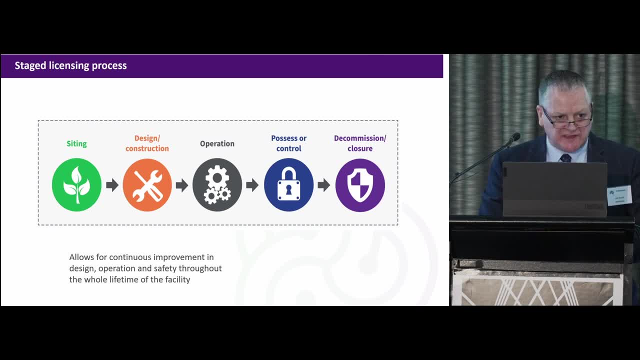 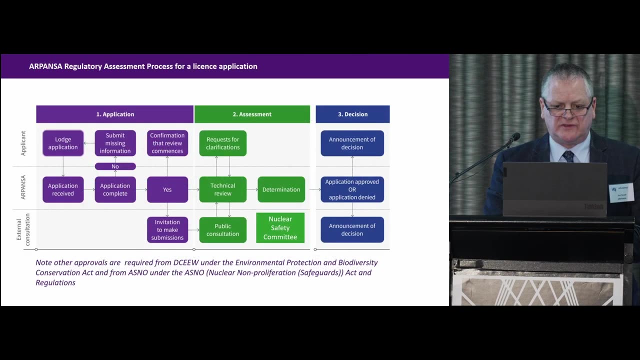 and having a staged licensing process allows the safety case to evolve throughout the life from basically from cradle to grave, as they say, And it's in line with international best practice. So this rather complicated slide tells you a little bit about our assessment process. 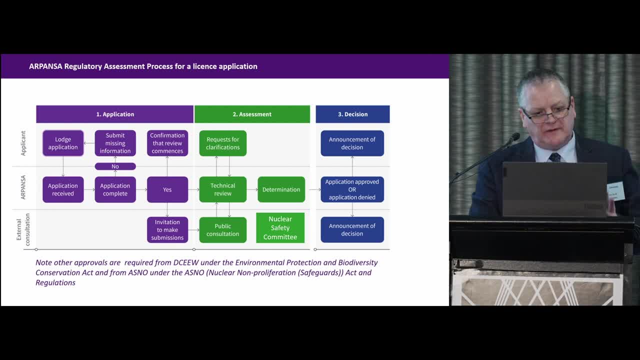 how we assess licences. So on the left-hand side you've got the application side, you know, and that's what needs to happen from the applicant point of view, Also Urpansa, what Urpansa needs to do. And then in the middle, the part in green, the part about 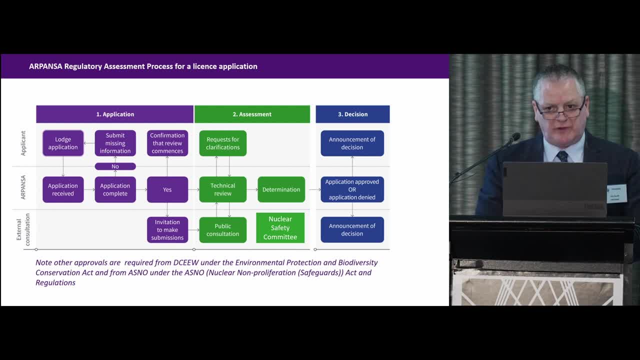 assessment of our applications And you'll notice here the public consultation. Now, that's extremely important. There is a requirement under our Okay regulations: If we licence a nuclear installation or a prescribation facility we have to undertake. 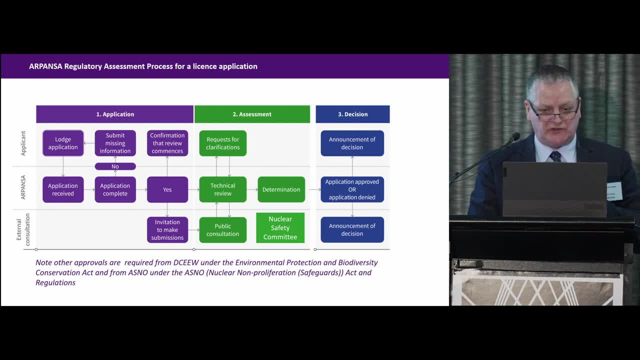 public consultation. Now the forum that I just mentioned to you that's happening on Monday is part of that for the HIFAR reactor, because it is a nuclear installation and it's at the decommissioning stage. We just received the application earlier this year, So we 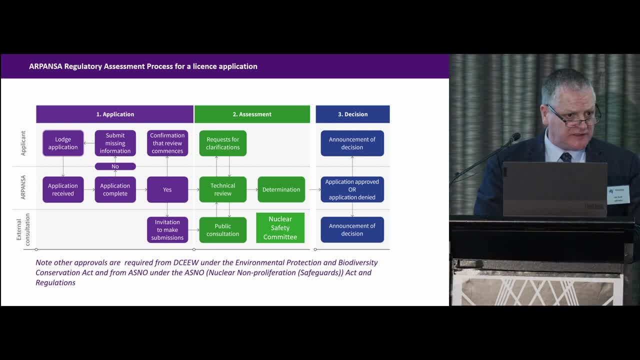 also seek, where needed, external advice, and we do that from our nuclear safety, So from our nuclear safety committee, and also through external experts we're required. We're not a large regulator so we don't have experts at every particular aspect of nuclear. 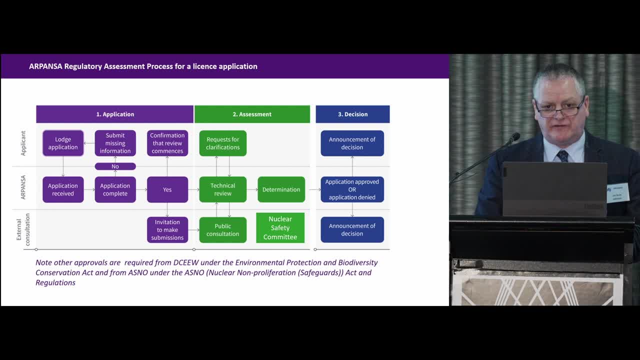 technology. So if we have a shortfall in that area, we can reach out to experts. So that's a little bit about the licensing process and right through to the decision- or in fact, you know, it could be an approval or it could be a rejection- Often during the course of 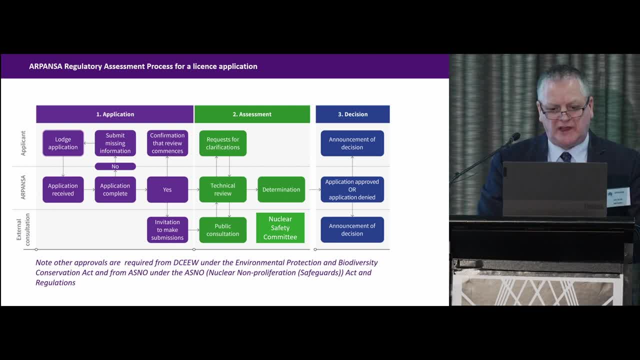 the application, we find there is information missing. So I'd like to point out this part. just above technical review request for clarifications, Often there is a back and forth between the regulator and the applicant to provide missing information with regards to the safety case. 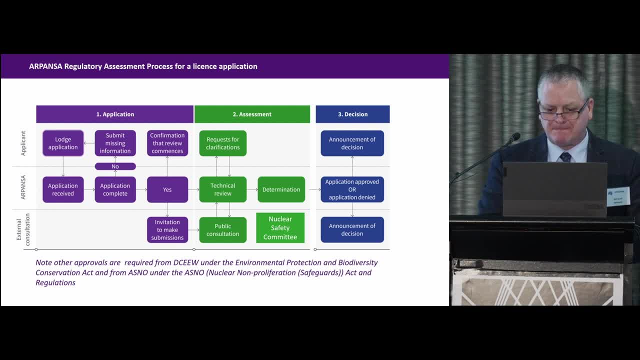 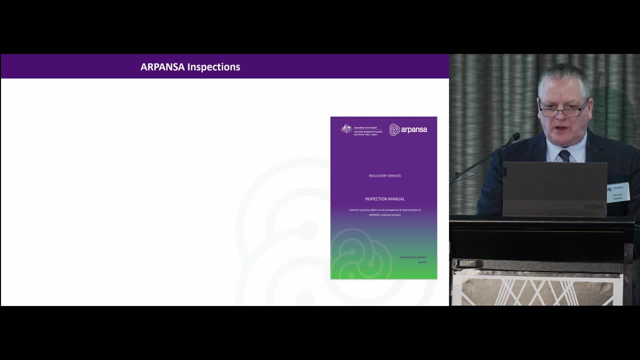 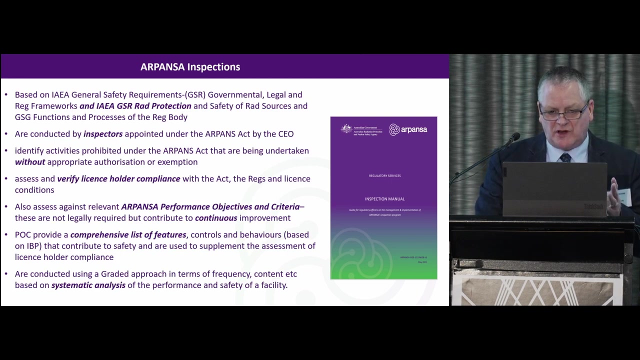 or to the application itself. Okay, inspection. So a lot of our information can be found on our website. It's actually under our inspection manual, right? and our inspection manual is basically based on IEA general safety requirements, one part, one which is governmental. 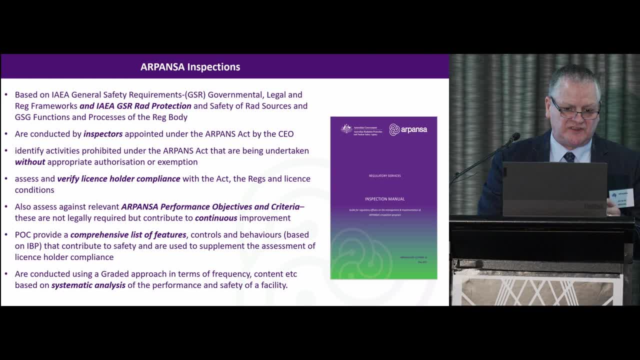 legal and regulatory frameworks and the IEA general safety requirements, part three, radiation protection and safety of radiation sources, and GSG 12,- sorry, general safety guide 12,, which is about functions and processes of the regulatory body. So all of our inspections are conducted by inspectors who are appointed under the ARPANS. 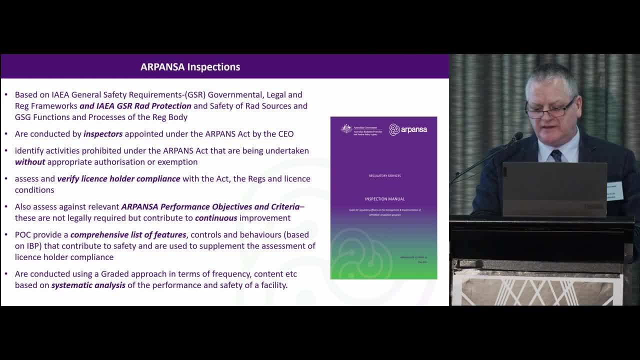 Act by the CEO, They have to undertake an intensive training programme to develop regulatory competencies. sorry, I didn't mean to do that so that, basically, that we have competency of inspectors and we have training programmes to achieve that. So what do they do? Well, 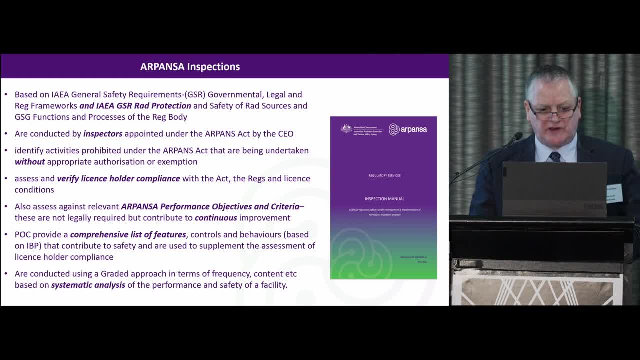 they'll undertake inspections to assess and verify licence holder compliance with the Act. We also have a set of what is known as performance objective criteria, which are not legal requirements, but they are guidance for our inspectors and for our licence holders. what we expect to. 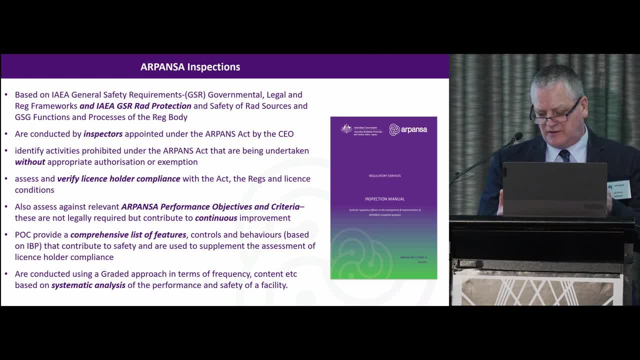 see in the course of an inspection. These areas cover inspection, testing and maintenance, radiation protection, waste management, security, emergency preparedness- the whole gamut of areas you would expect to see at a nuclear installation. So they are conducted in a graded approach. we do them for prescribed radiation facilities. 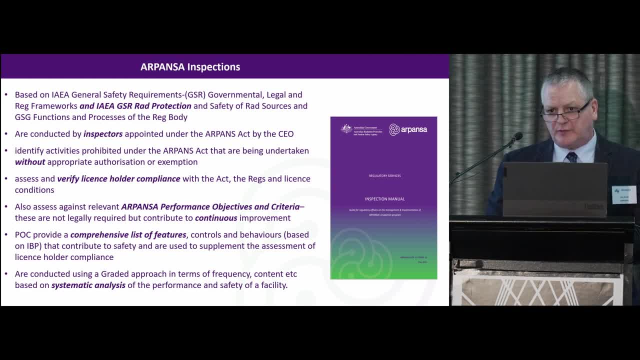 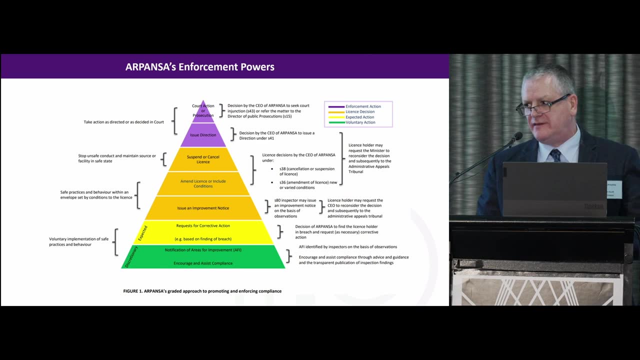 like linear accelerators or radioactive waste stores, but it's a graded approach. obviously you expect less from an inspection of them than you would for a nuclear installation, say of a research reactor. And enforcement right now, this rather complicated regulatory pyramid. 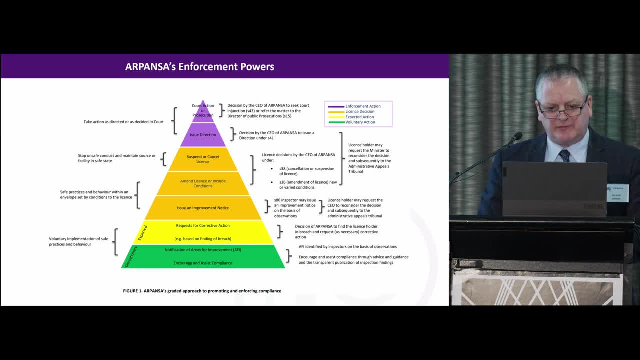 So this is a standard. This is a standard way of expressing a graded approach to enforcement amongst regulators, Starting from the bottom. we have the green area, which is encouraging compliance and also notifying licence holders of areas for improvement to achieve best practice up to 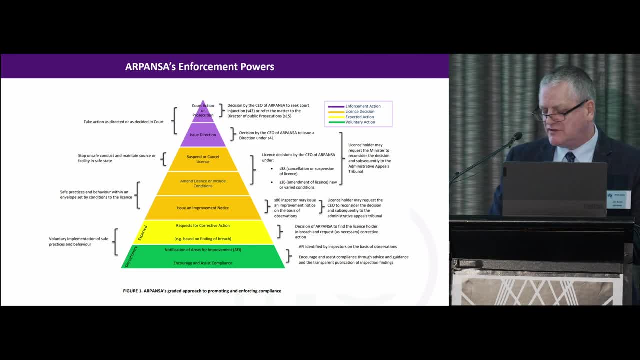 the top where you have court actions and prosecutions. Fortunately, we've never had to go there. we've never undertaken a court action or a prosecution. We've noted that all of our licence holders are government agencies and they generally tend to be compliant and they will generally rectify areas for improvement fairly quickly. 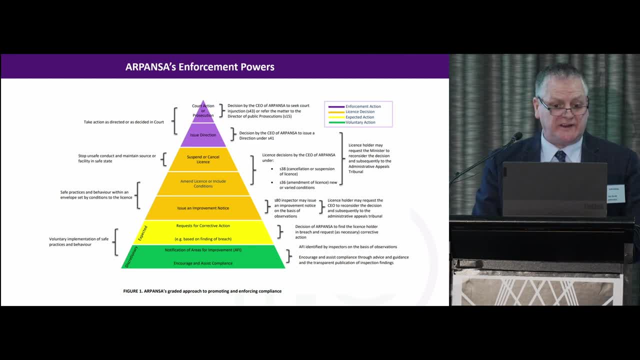 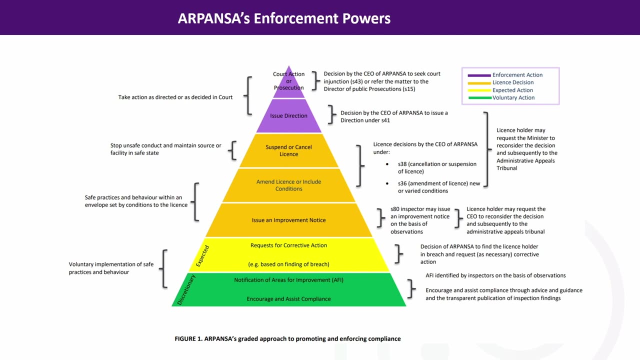 and so we've never had to go to the legal prosecution of any of our licence holders. In the middle, the mustard-coloured steps are where we tend to be in our compliance, and that includes issuing improvement notices, amending licence conditions Or adding amending licences or adding licence conditions, which is very common actually. 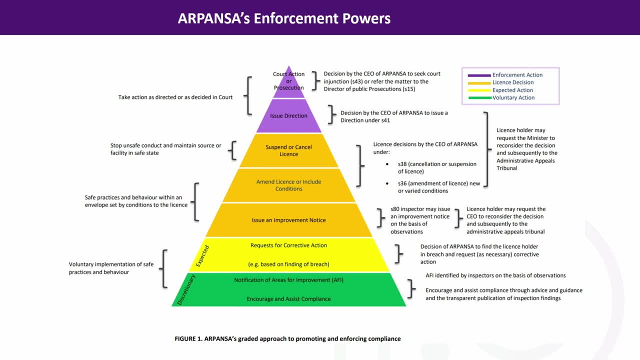 for our enforcement where we find deficiencies in the operations of our operators. And there's also suspend or cancel the licence. Again, we have not had to do that in our history, our 25-year history of suspending or cancel licences. 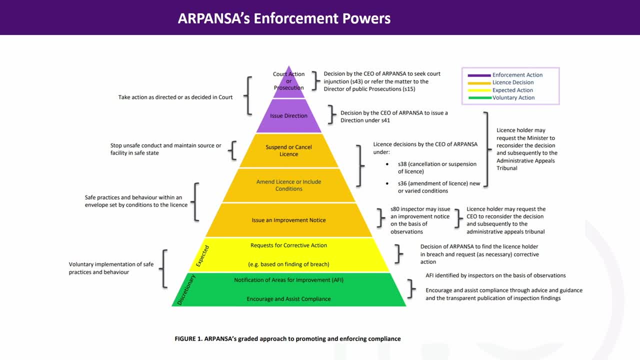 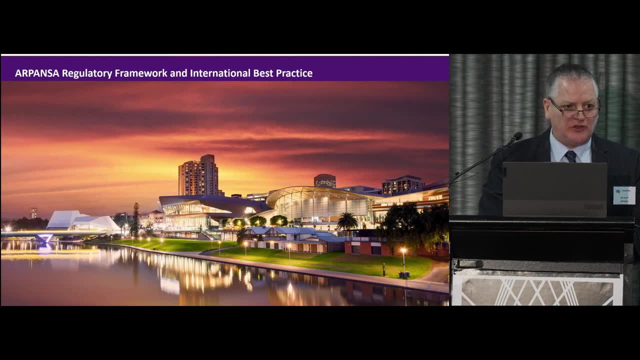 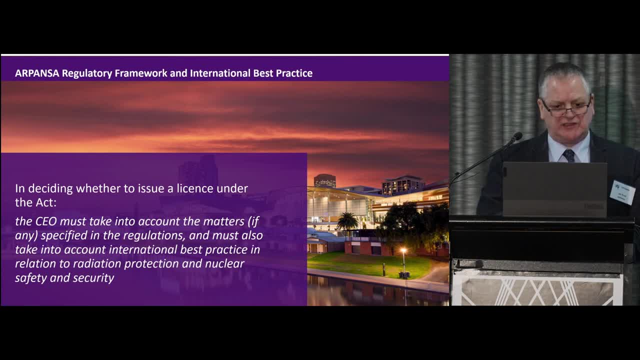 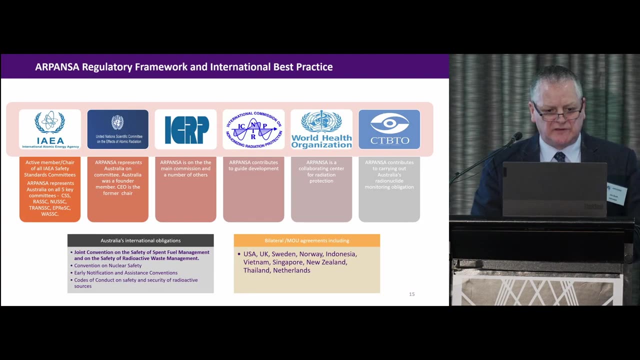 So it's in our Act and Regulations that we- well, it's actually in the Act- we- must take into account international best practice in radiation protection and nuclear safety and security. And how do we do this? Well, that's interesting. So our PANZA has got a lot of engagement with international agencies such as the International 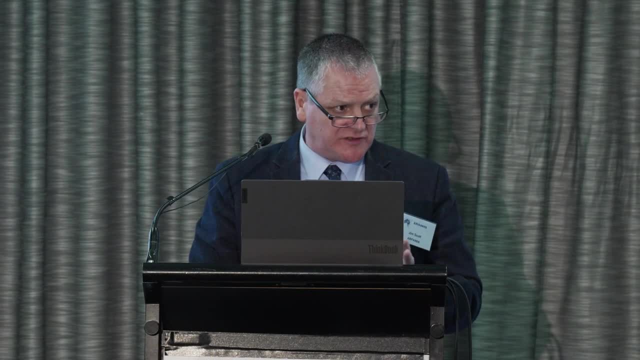 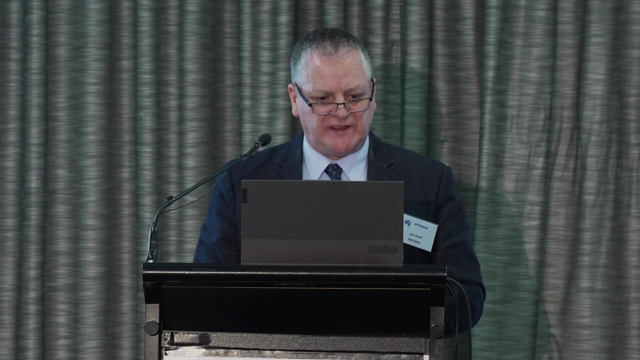 Atomic Energy Agency. In fact, we've represented in all the major safety standards committees, such as the Commission on Safety Standards, the Radiation Safety Standards Committee, the Nuclear Safety Standards Committee, TRANSC, the Transport and Nuclear Safety Standards Committee and EPRESC. the 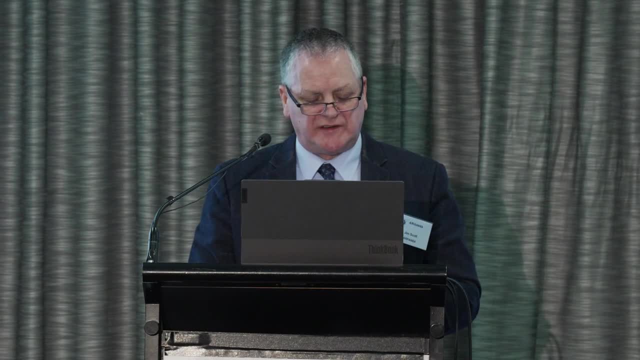 Emergency Preparedness and Response Committee and WASC, the Waste Standards Committee. By doing that, we are kept a brief of what is currently best practice in areas of radiation protection and nuclear safety, In all of these very important areas. that is not the only one, of course. that is UNSCEAR. 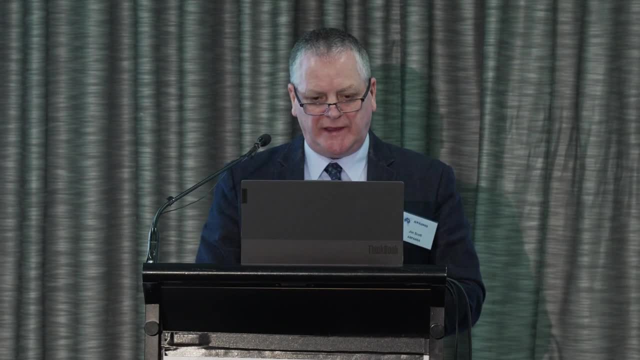 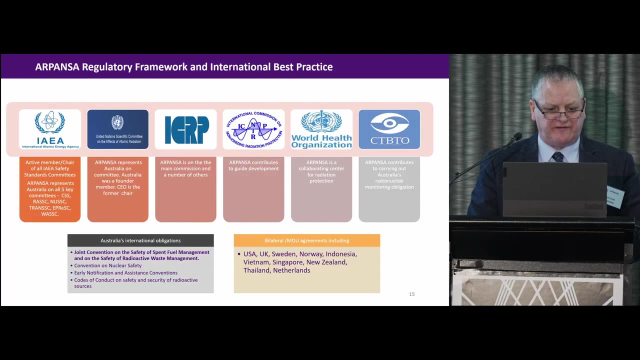 which does undertakes research for the harmful effects of radiation to people, And in fact our PANZA, or Australia, is one of the founding members of the UNSCEAR organization. Then, of course, there's the ICRP, the International Commission on Radiation Protection. 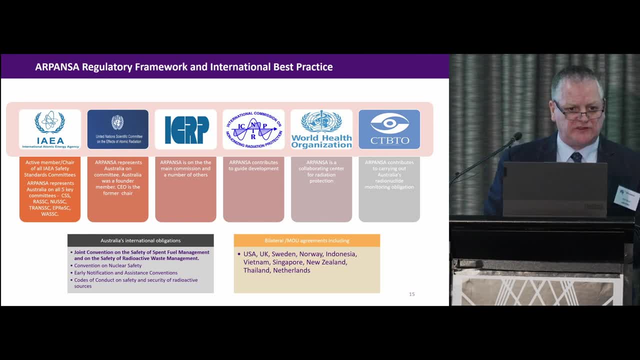 Now the next one is a little bit unusual: ICNRP, which is International Commission on Non-Ionizing Radiation Protection. We are one of the few regulators in Australia that actually regulates non-ionizing radiation, So that by that we mean powerful lasers, UV, radio frequency, microwave- sorry, she's. 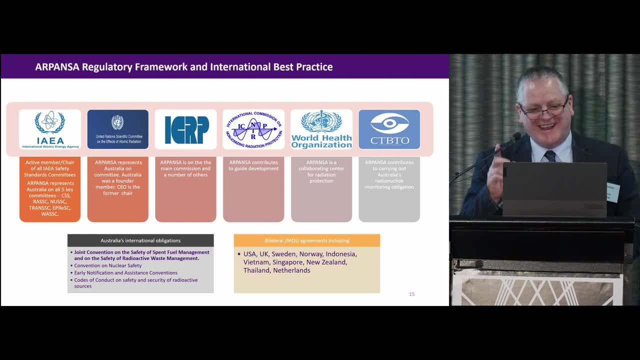 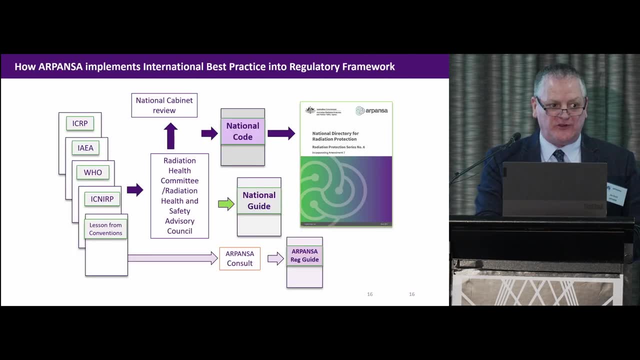 approaching me- I'm almost there, so don't worry- and World Health Organization and the Comprehensive Test Ban Treaty Office. So how do we do it? Well, we write codes and standards and we do it through this complex slide through our Radiation Health Committee, which is actually established under our Act, and it comprises: 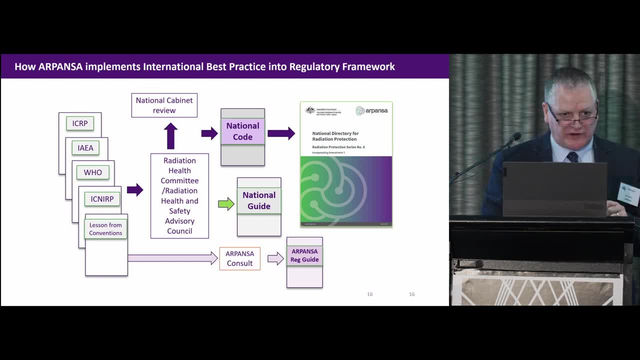 senior radiation control officers from each of the state and territory regulators and, of course, our PANZA, And we produce guides on radiation protection and nuclear safety and these are published on our website. So that's how we do it. So conclusions. 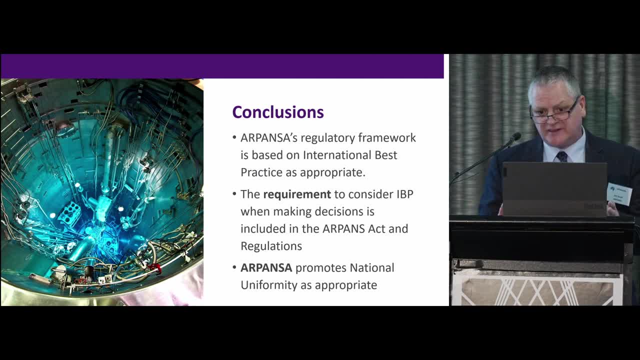 So our PANZA's framework is based on. It's based on international best practice as appropriate, and the requirement to consider international best practice is actually written into our Act and regulations, and we promote national uniformity where appropriate. I should have pointed out one of the CO's function is to promote national uniformity.